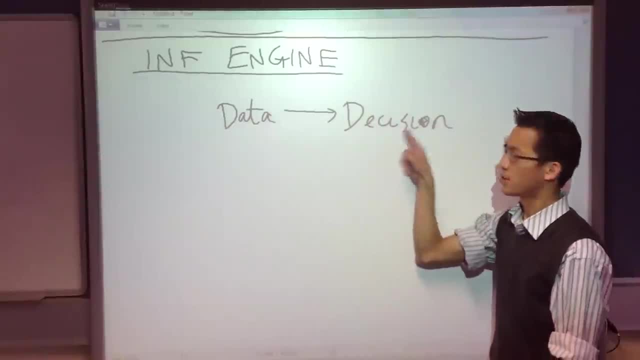 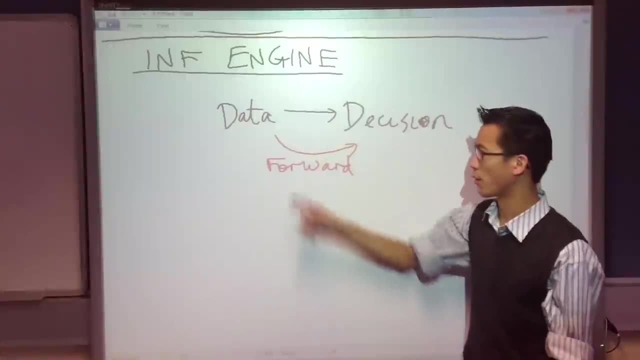 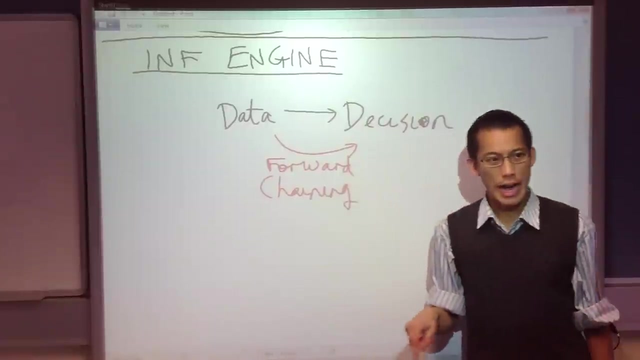 way, let me give you names on this and then I'll try to explain it. Going from data to the decision: okay, it's called forward changing Because, as is implied, you're going forward from data to the decision Now. you may, or the system may, start from a decision and go back towards data Now. 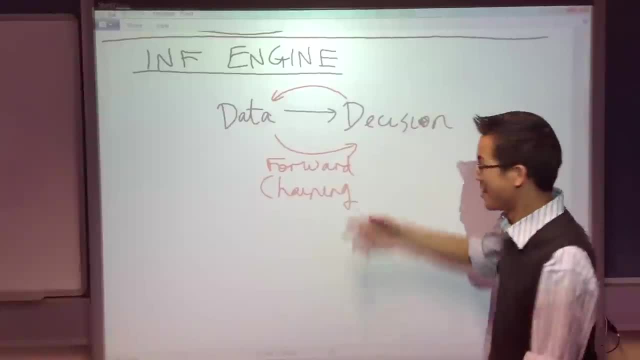 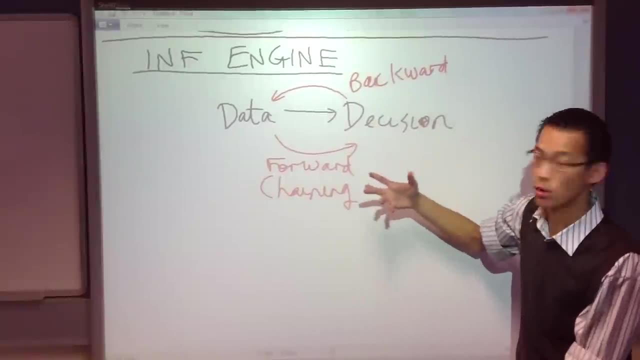 that might seem a bit backwards to you, which is why it's called backward changing, But actually, as you'll see in a minute, as humans we use both of these on a regular basis all the time. My question is trying to imply this, right. 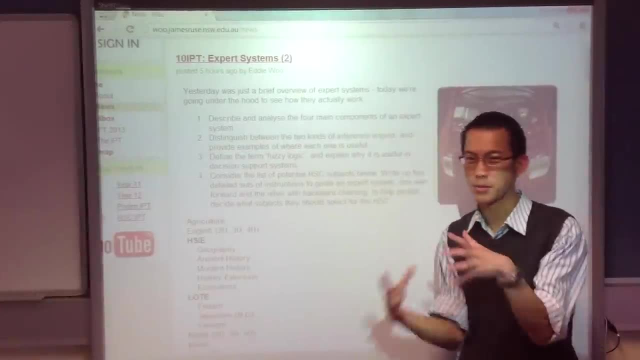 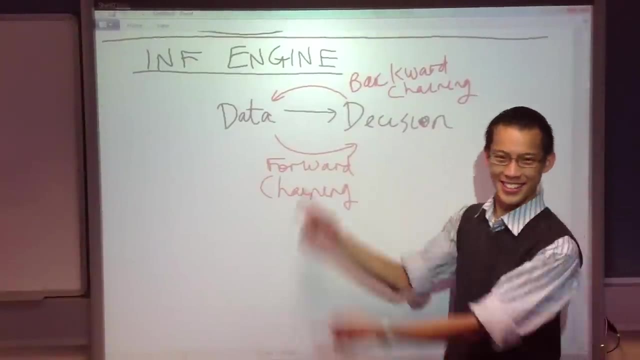 Sometimes one is useful and sometimes the other is useful, and sometimes a combination of both. So let me try and explain. So do you think backwards? I'm going to start with backward changing. okay, Backward changing. Now the idea is, I want to make some kind 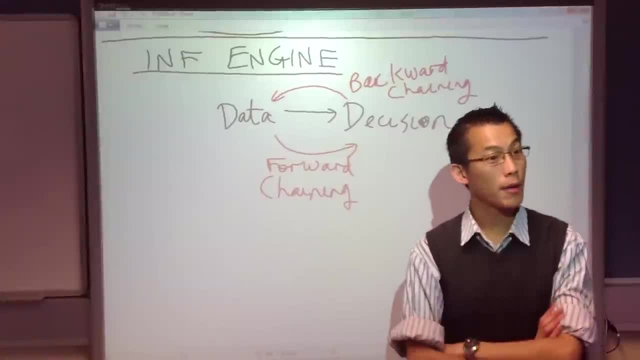 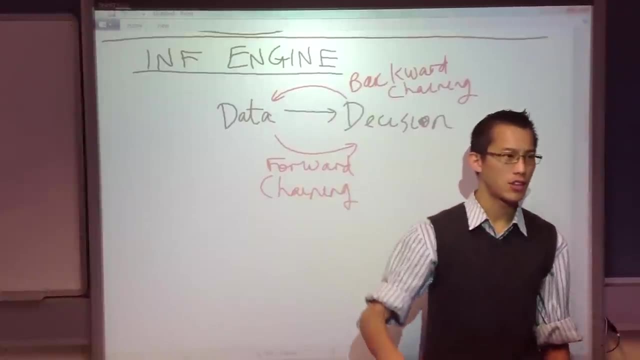 of decision, right? So I think I was talking about the weather before and whether I should wear an extra jumper. okay, Now pause there for a second. I get up in the morning and I'm turning the lights on and I'm about to pick some clothing. okay, Now that question. 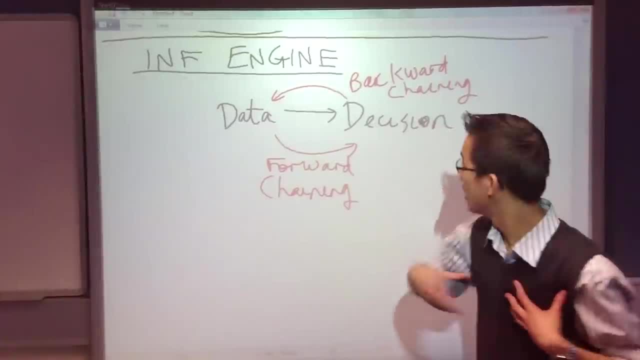 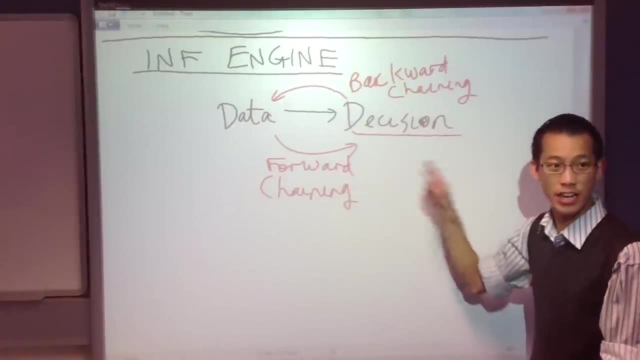 should I wear a jumper, an extra jumper, today? right, That's the decision, right? So actually, my starting point, the starting point of my thinking, is: here's a decision and I want to know whether I should do it or not, or what kind of variables there are. there like: 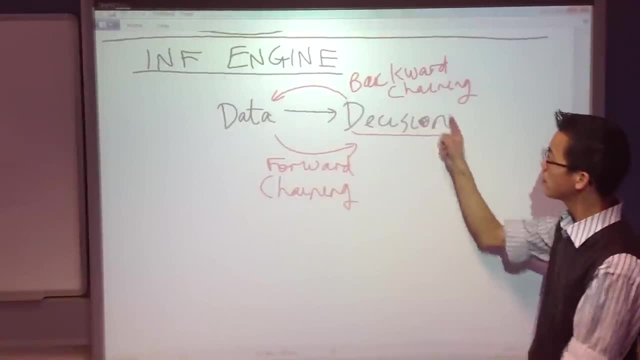 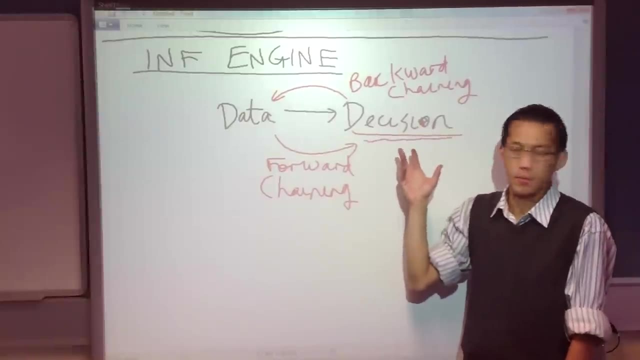 which jumper should I wear, something like that. So in that case, I've actually begun here. on this side I'm backward changing, right. So now that I've started with my decision, I need to see should I do it or not. So now I've got to go search for some data that 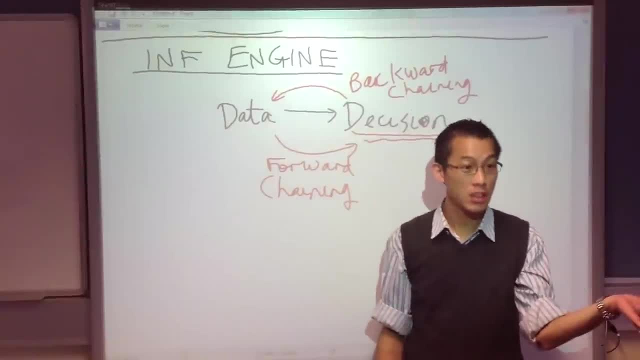 relates to that. So I've got my phone out and I check the weather, right, Or you know, Wi-Fi is down or something like that. So I look out the window, I open it up and I'm like, is the? 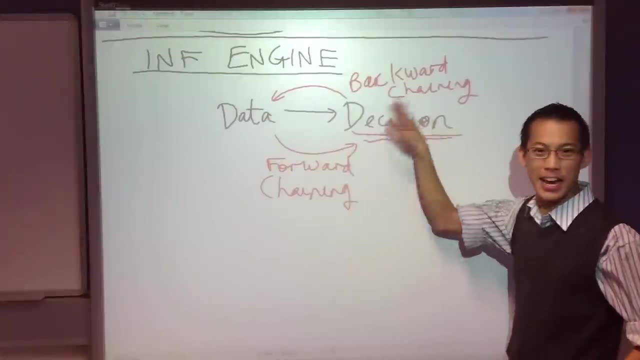 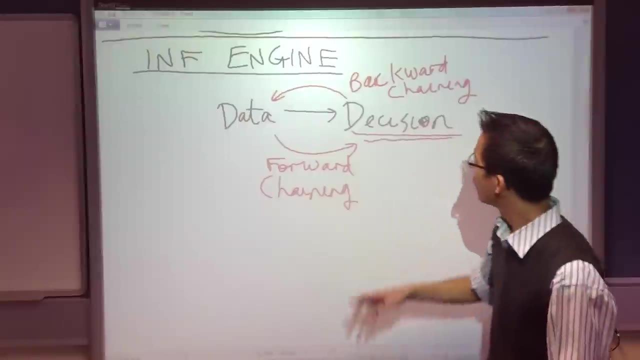 air coming through, cold or not, right, So you can see, starting from this decision, it guides what data I should look at. Does that make sense? So in some ways you might think of this as a convergent approach, right, I've sort of got a goal in mind and I'm sort 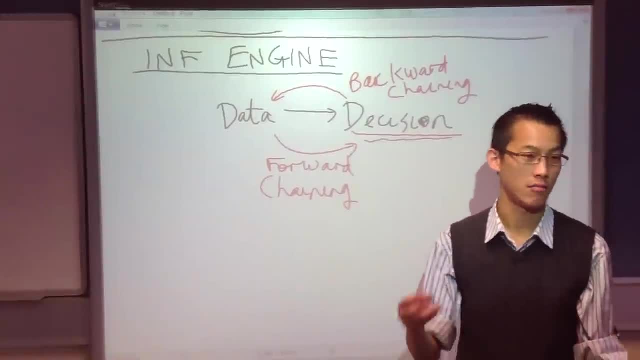 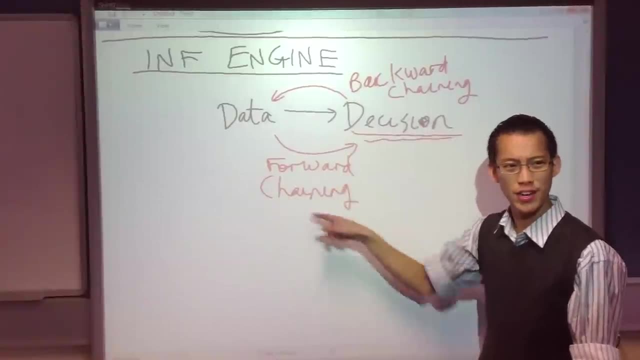 of drilling towards that, And once I've got enough information, then I don't need to look at anything else. So I make my decision. That's backward changing. How does forward changing go? Well, as the name implies, you don't start with the decision you're going to make. You might have no idea. 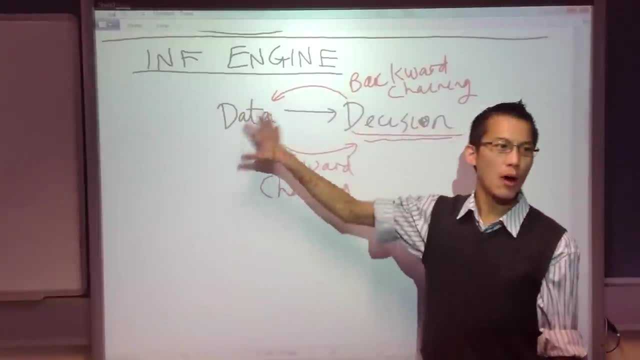 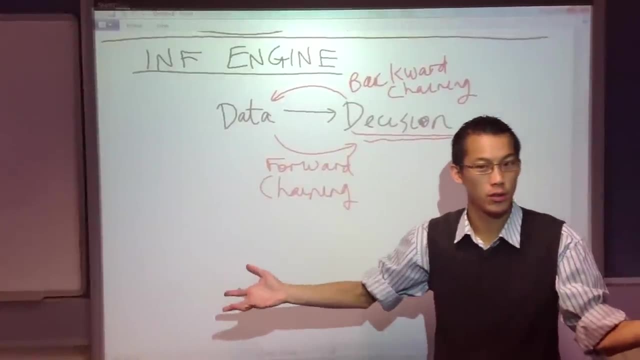 what decision you're going to make. okay, Instead, you just start with the data. What do you know? right? Gather as much data as you can, Just get everything. You don't know whether it's going to be relevant or not. Just grab it. okay, Once you've got all of. 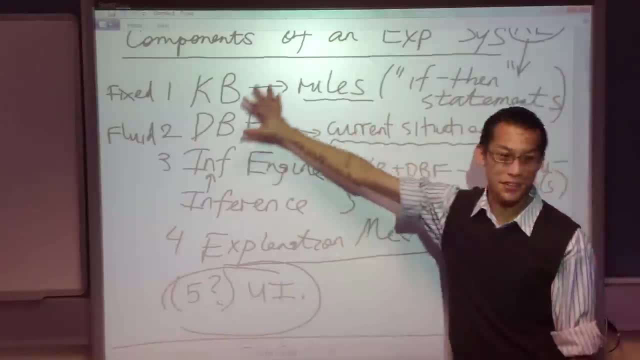 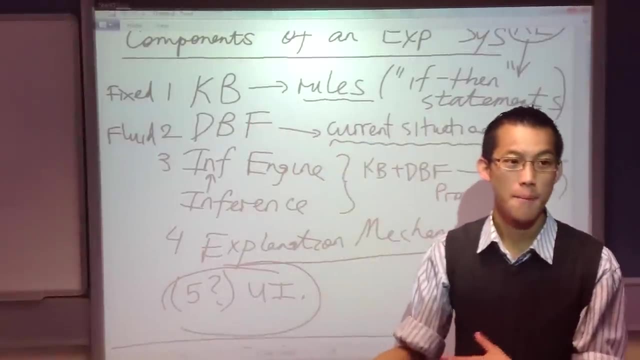 that try your best, Combine everything you've got, You've got here right And see all right. what does this lead to? What decision or decisions might this lead me toward right Now with the clothing? that wasn't such a good example. 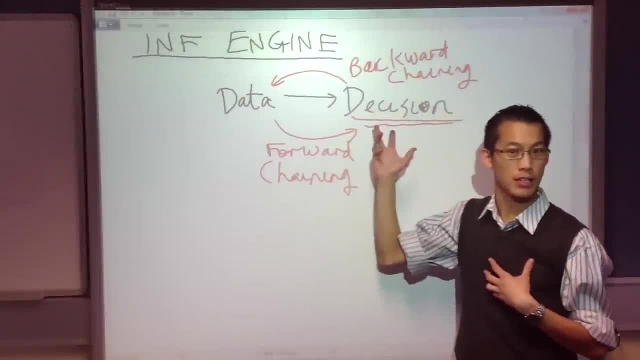 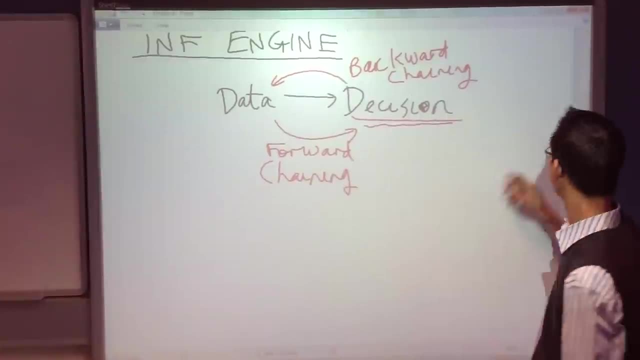 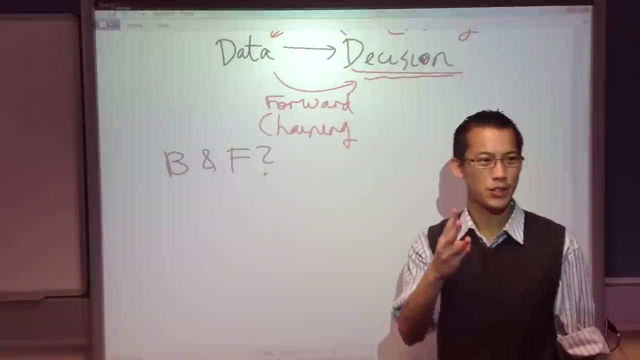 for forward changing. That was more of a backward changing situation. Start with the decision: look for some data. okay, But just yesterday I had to make a decision which was forward changing, which was: who should I choose to be the three people to get the most data from? 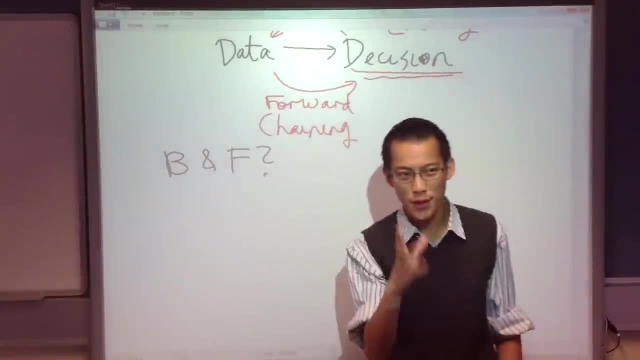 But I think that's a good example. I think that's a good example of how to do a free decision, And so I'm going to show you guys how to do this. So I'm going to show you guys how to do this. I'm going to show you guys how to do this. So here's what we're going to do. We're going to do a free decision. We're going to get points for best and fairest after sport, okay, So if you don't know, the system best. 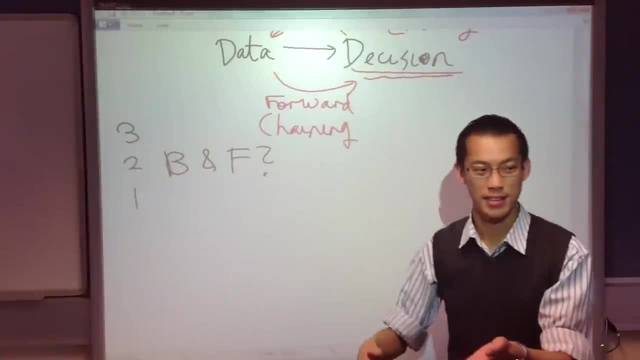 and fairest for great sport. you don't just pick one person who gets the award, you actually pick three And they get three points, two points, one point okay, And at the end of the season you add up everyone's points and then you get an overall best and fairest. 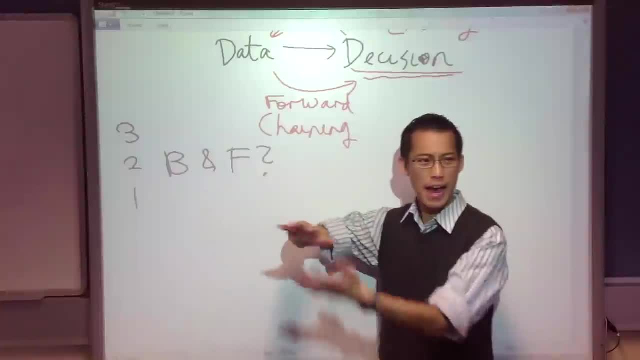 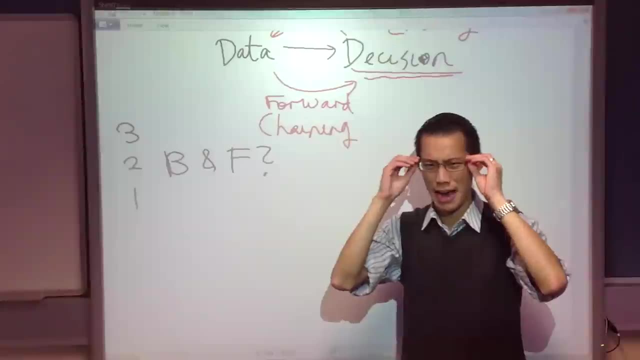 okay. Now here's the thing: I have 24 people on my two teams. Actually, I only had 12 people who played a game yesterday because, unfortunately, our Bs didn't. Our Bs were so awesome, they intimidated the other team and they didn't even turn up, So I just had 12 players to choose from. 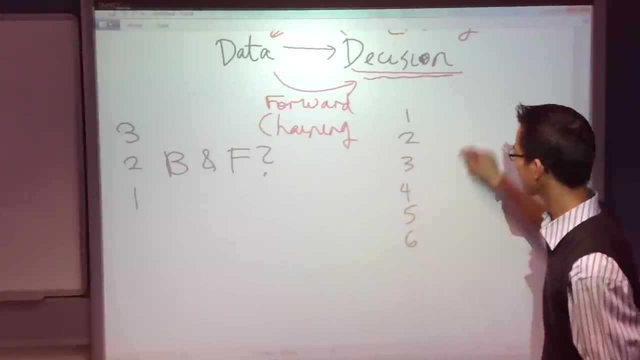 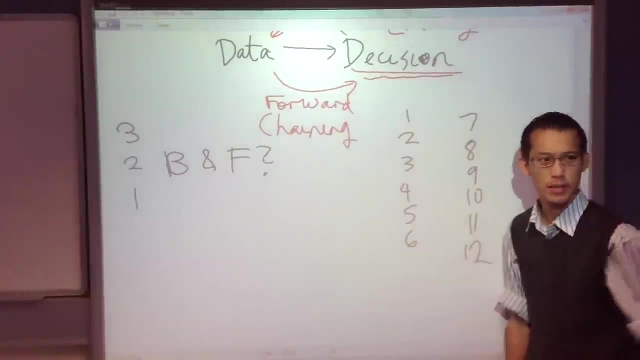 So I go and I look at my list. Now, if I were to backward chain this, it would look something like this: Look at player number one. Should this person get points for best and fairest? So there's my decision that I have to make. 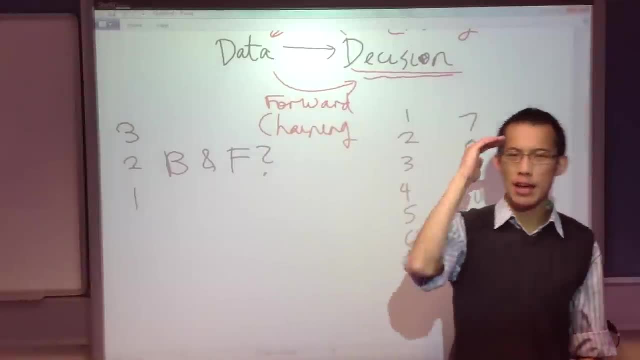 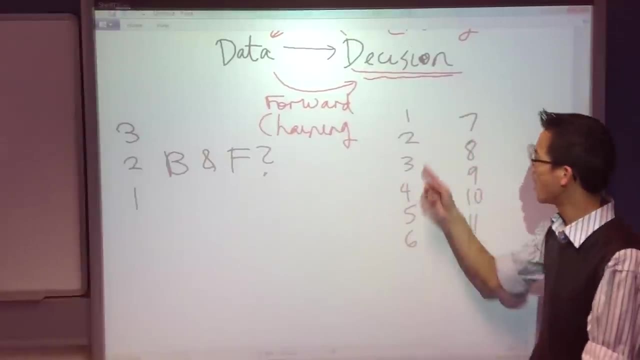 And then I think about what data relates to that. So then I think back through the game. I'm like, oh okay, they did this. oh, they dropped the ball there. oh, they scored there, and so on. So then I will think, okay, now that I've got as much data as I can, I'll make a decision. 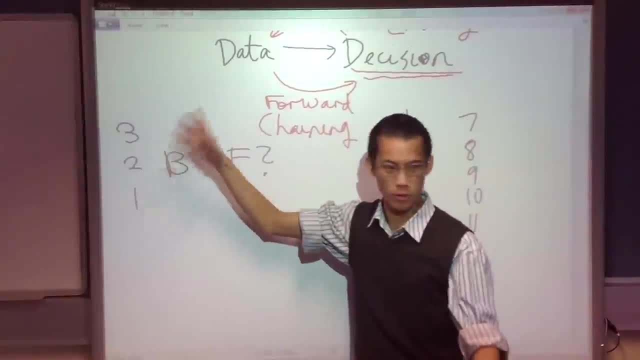 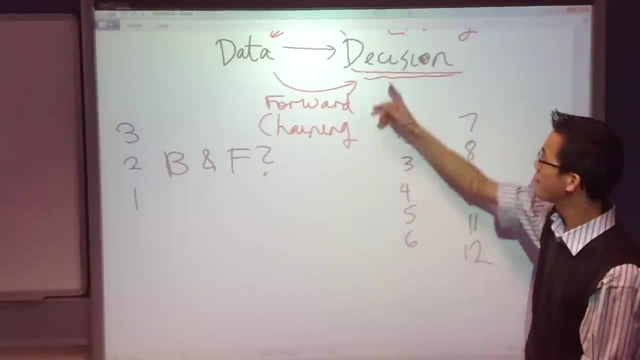 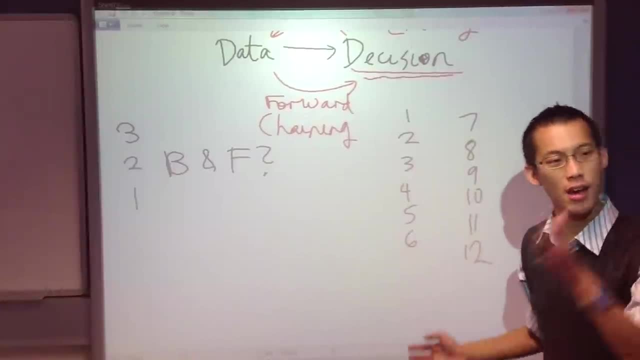 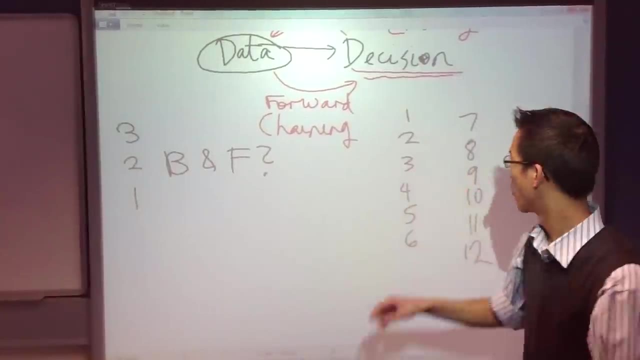 It's a very time-consuming process in this example, So instead I'm going to start with the data. I'm going to now go back to the game first, rather than any particular decision, And replay the game. I'm like: okay, this is what happened. 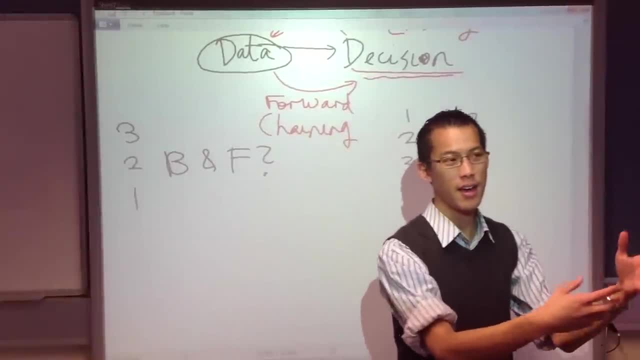 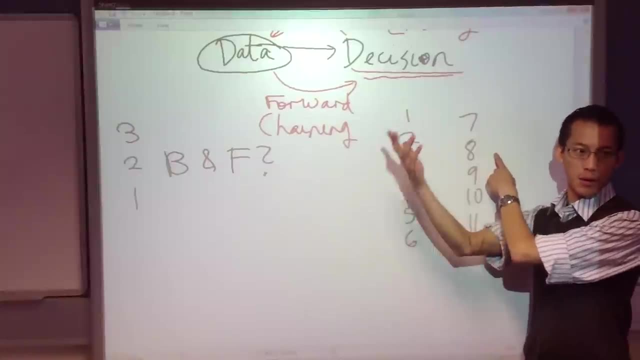 This is what stood out. This was unusual, This doesn't usually happen And I'll think- okay, based on all of that data, I'm going to make a decision- that this will be a person who I think stood out the most. 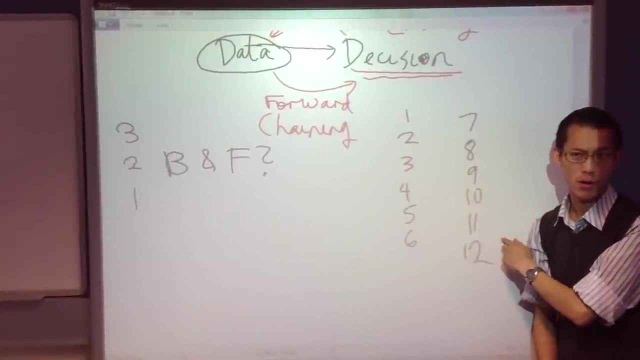 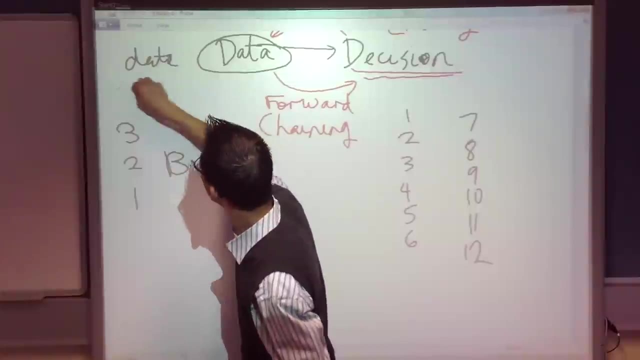 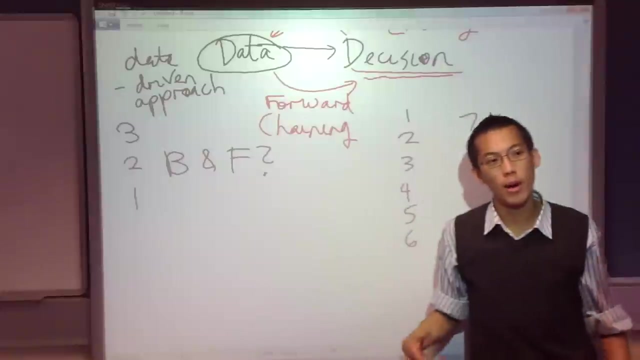 And they're going to get three points. This one will get two, This one will get one. So, because it begins with the data, this is often called a data-driven approach. It's often what works best When you simply don't know which choices to actually start asking right. 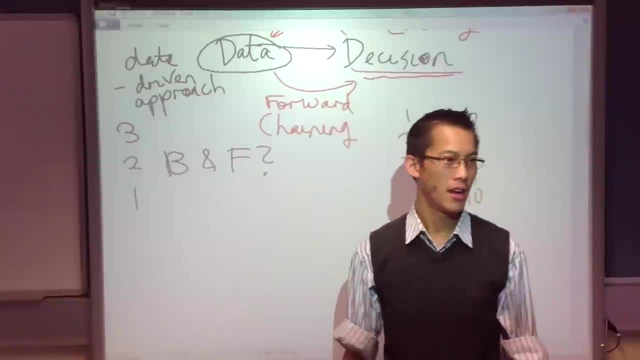 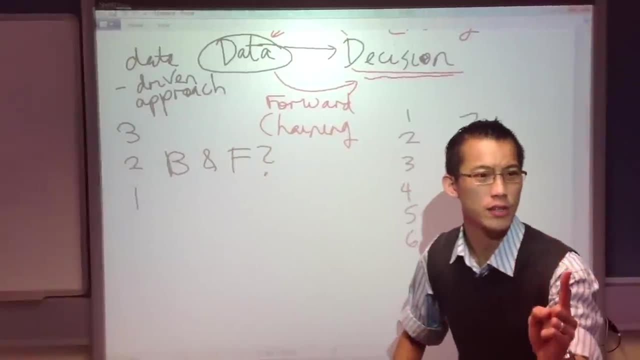 All you can do is look at the situation and say, well, what do we know And therefore, what decisions can we make on the basis of it? right, It's often also very helpful where there's not just one thing you have to choose. 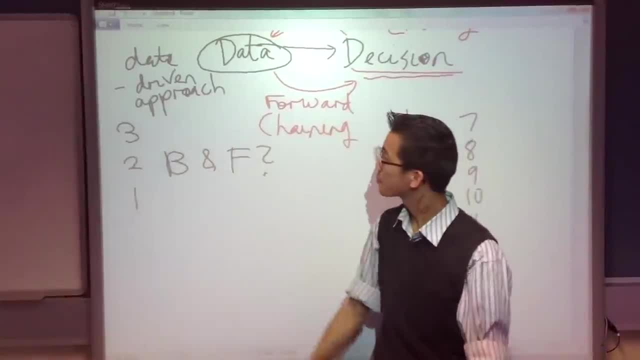 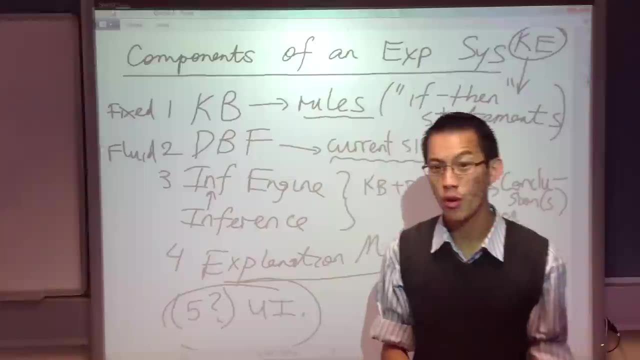 You're actually going to end up with a few different conclusions, right? So, for instance, in my knowledge base, my rules might be things like: if someone scores, right, I look at all the people who scored. Well, maybe I have three players. 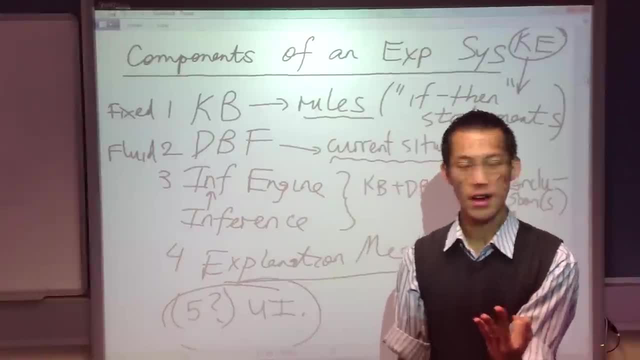 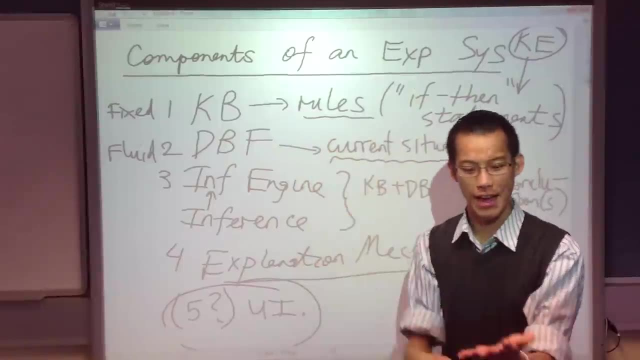 And I'll say, okay, they're going to be my top contenders for best and fairest right. So there's a rule that's fired, that's been related, that's been relevant right, And then I'll have a look at other rules and I'll put that all together and I'll see who are my top three. 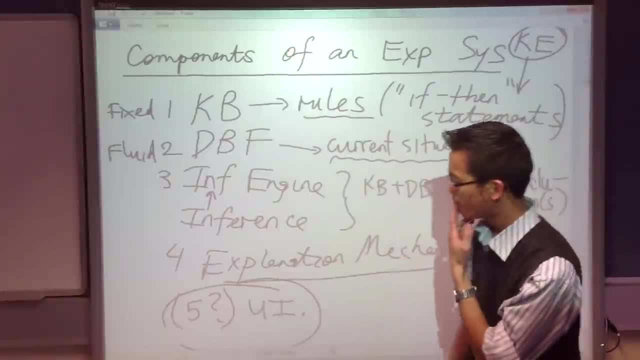 So you see how it's a different way of looking at it, right? Does anyone want to clarify on any of that?